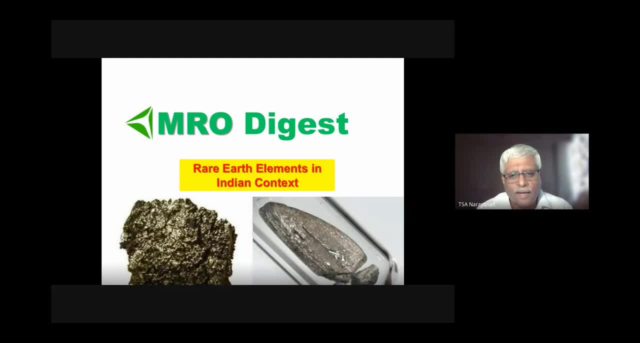 can't actually call it rare earth, But the terminology was given long back, So we are continuing with that terminology as such. Otherwise it's available in plenty. With this as the background, I will cover my presentation at the following: aids Introduction application. 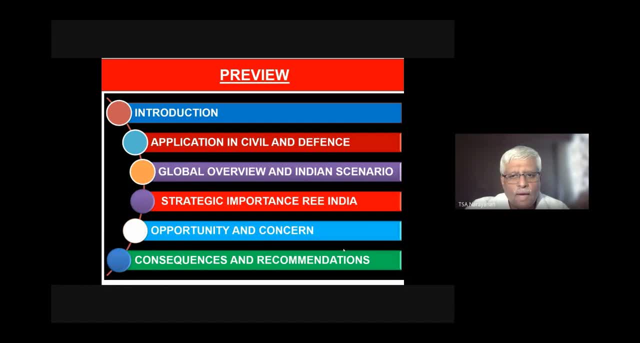 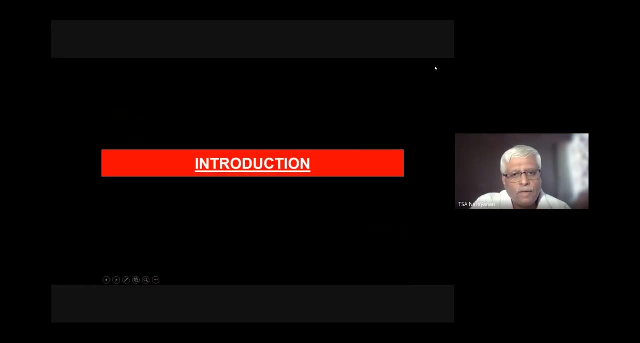 and civil and military. global overview and Indian scenario. strategic importance of rare earth elements in India: the opportunity and concern for us, the consequences and recommendation. Coming to the introduction, you are all familiar with this. This is the periodic table. If 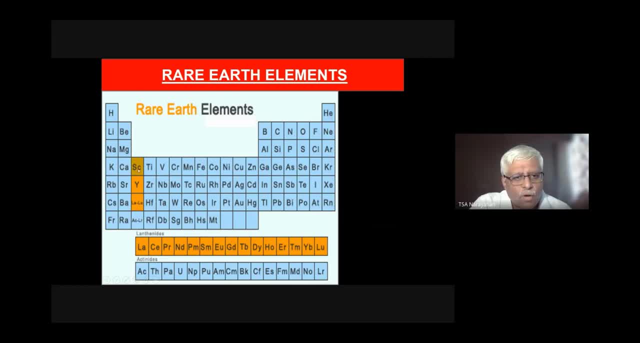 you look at on the screen, this SC which I am pointing through my mouse, and Y are the rare earth and this LALA. The expansion of LALA. are these lanthanides, These 15 lanthanides, and these two, cerium and ethereum. they constitute the rare earth as on date, These rare earth. 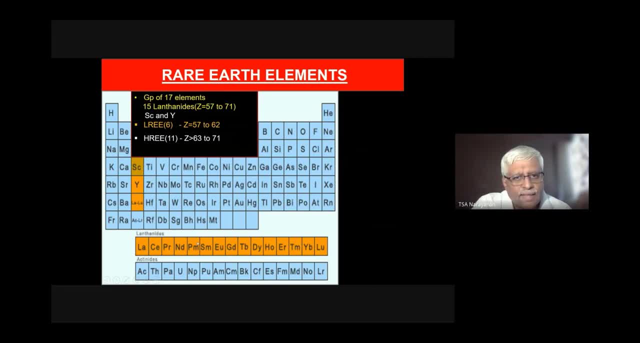 are a group of 17 elements, out of which 15 are the lanthanides, from atomic number 57 to 71, out of which the lower rare earth element- and I say low rare earth element- are this LA to SM, These actually in the rock, their content is very low. So extraction process. 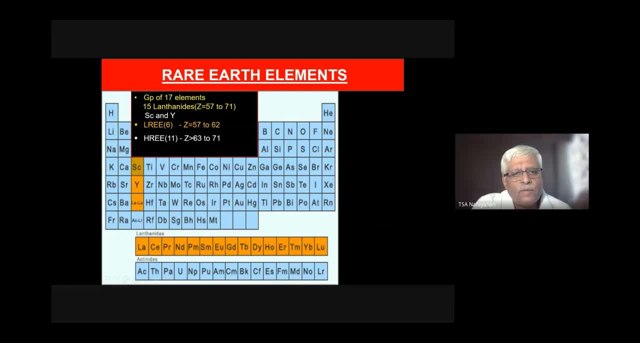 is more cumbersome, Whereas the higher rare earth are from Z 63, at the atomic number 63 to 71,, starting with Urut, Europium till Etorium. Now, if you look at, what are these rare earth elements? these rare earth elements, if you? 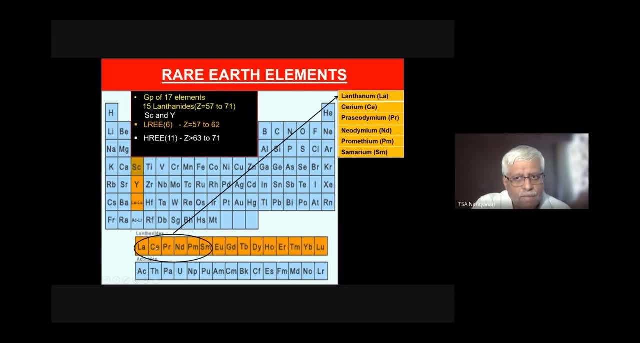 expand. they all stand for Lanthanum, Cerium Trisodium, Neodym, Promethean and Samurai. they all look green. Are these elements? Are these elements this red? Are they two green? Are they two yellow? 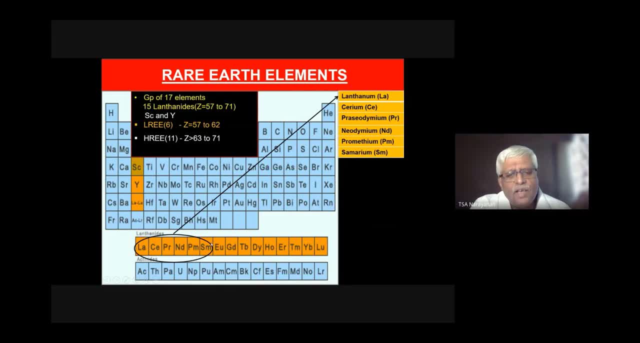 Are they two orange? Are these two yellow? Are these two yellow? What are they? Are they two? agreed to us in terms of the way, but they were all derived at the place either some have been named over the city, somewhere named over the scientist name, something like that. 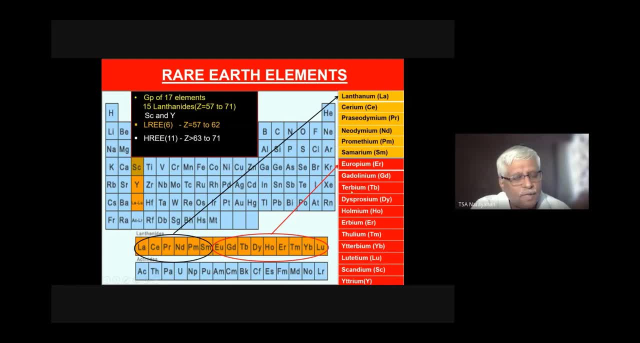 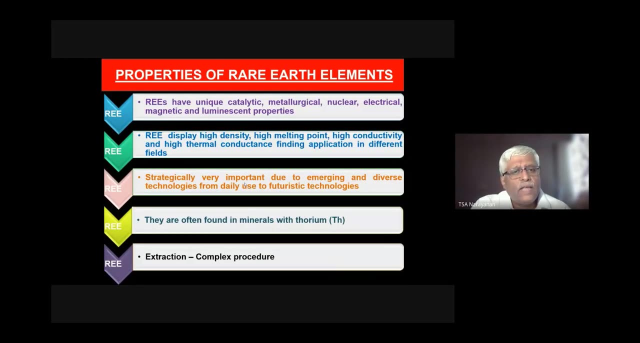 the higher rare earth are the europium, gadlonium, terbium, dysporium, aluminium, erbium, thulium, ytruvium, lutetium and scandium and uterium are the sc and y. what are the properties of rare earth? they are unique catalytic, metallurgical, nuclear, electrical, magnetic and lumison properties. 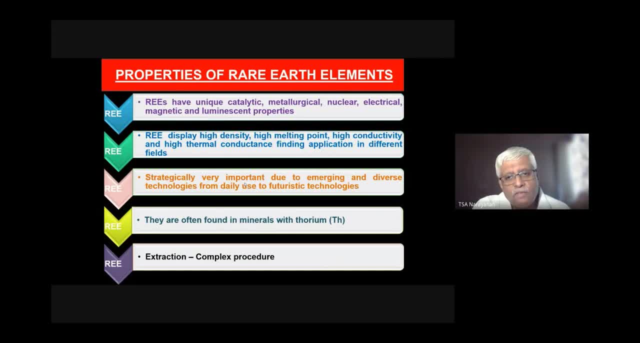 very rare to have a metal like this which has got so many properties. so they display high density, high melting point, high conductivity and high thermal conductance, finding applications in different field. they're strategically very, very important due to emerging and diverse technology, from daily use to futuristic technology. 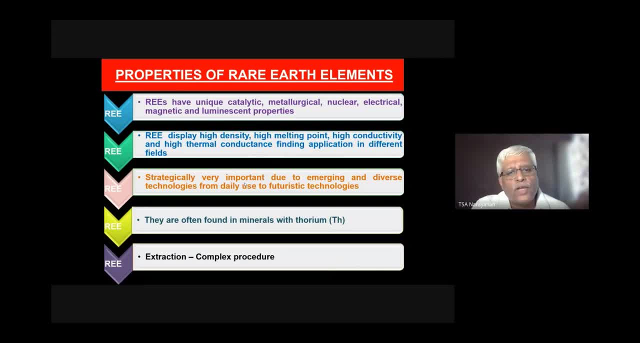 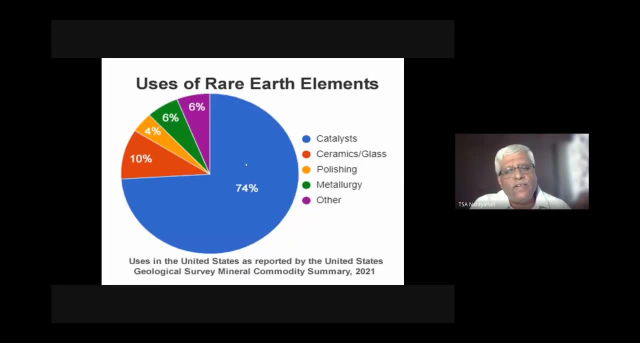 they are always found in minerals with thorium and the extraction, i said, is a very complex procedure. it is easier to extract hre, that is, the higher rare earth elements, than the lower rare earth elements. what are the application in civil and defense? so come to starting with. 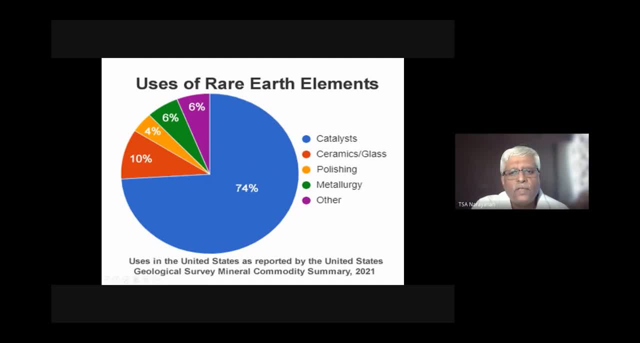 a civil application. if you look at this graph, the 70 percent of rare earth is used for catalyst. i'll explain this later. 10 percent is used for catalyst and 10 percent is used for catalyst and 10 percent is used in ceramic complete glass manufacturing. 4 percent is for use for polishing, 6 percent. 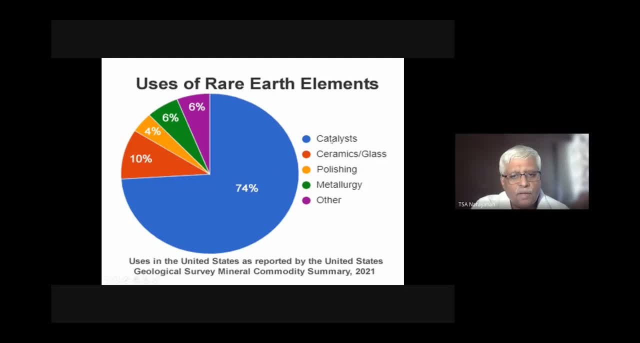 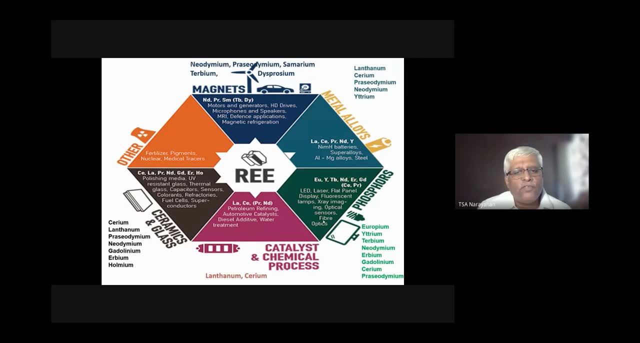 is used in metallurgy and others are 6 percent, if i expand it further. this, this slide, gives you the complete usage of rare earth element as such in civil application, starting with magnets. these are the rare earth which get used in making of magnets. these are the rare. 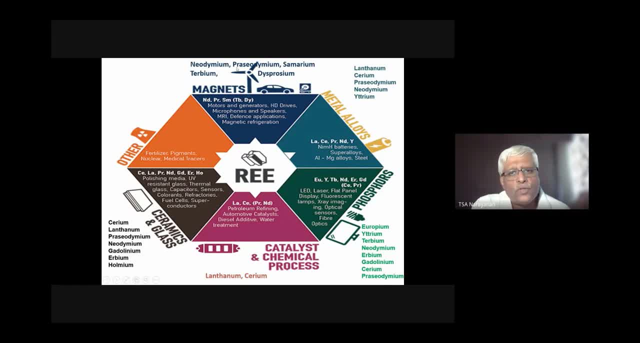 earth permanent magnets, that is, the neodym presodium, samurium, terbium and dysporium. where are these rare earth magnets utilized? they are utilized for motors and generators, hd drives, microphones and speakers, for mri scan, various defense application and in magnetic refrigeration. coming to the metal, 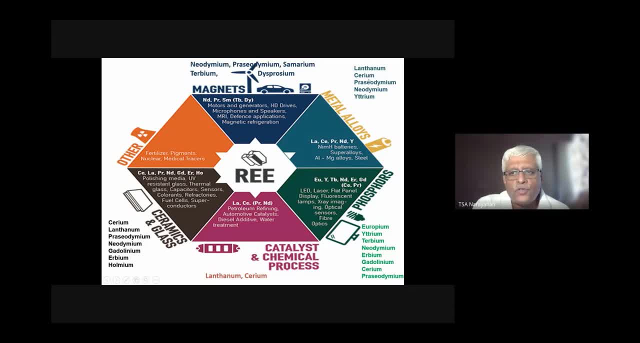 alloys you have the lanthanum, cerium, presodium, neodym, uterium used for making the metal alloys, also used for nimh batteries and super alloys, aluminum, magnesium alloys and in steel manufacturing used as phosphorous, where the europium, yttrium, terbium, neodym, gindolium, cerium and presodium are used in. 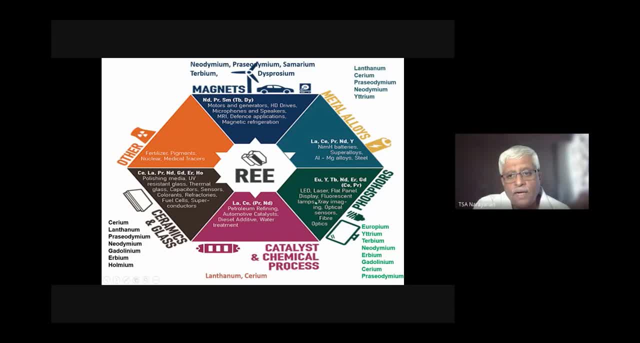 manufacture of leds, laser flat panel, flat panel display, fluorescent lamp, x-ray imaging, optical sensor and fiber optics. as i said, 70 percent is used for catalysts. these are the catalysts and chemical process. what is used is lanthanum and cerium, along with prosodium and neodym. they are used for petroleum refining. 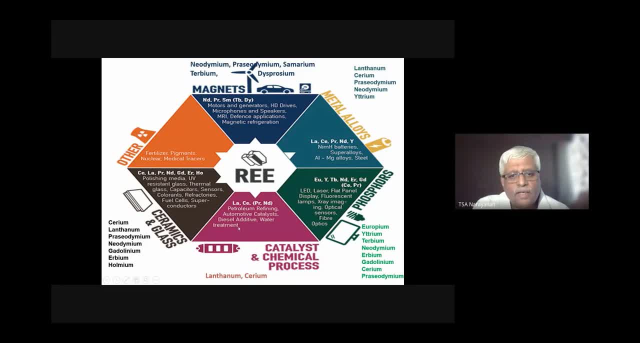 automotive catalysts. one of the catalytic converter also has this decelerative and water treatment, and in ceramic and glass you have cerium, lanthanum, prosodium, neodym, endolinium, erbium and aluminium being used for polishing media ultraviolet resistant glass. 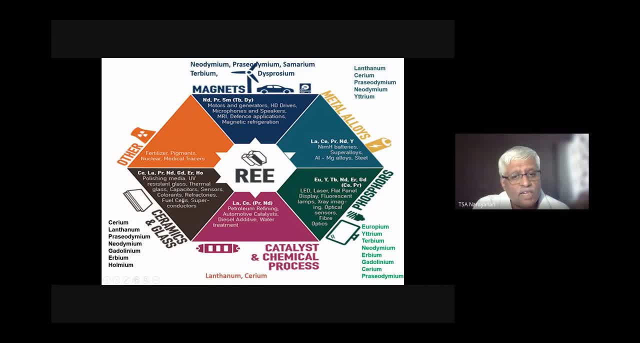 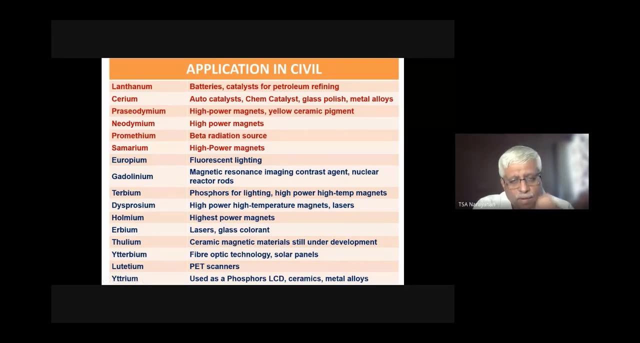 thermal glass capacitors, sensors, cool colorants, refractories, fuel cells and superconductors, and others are used for fertilizers, pigments, nuclear and medical tracer. coming to proper application, bit by bit- i mean rather element by element- you can have a look that the first six. 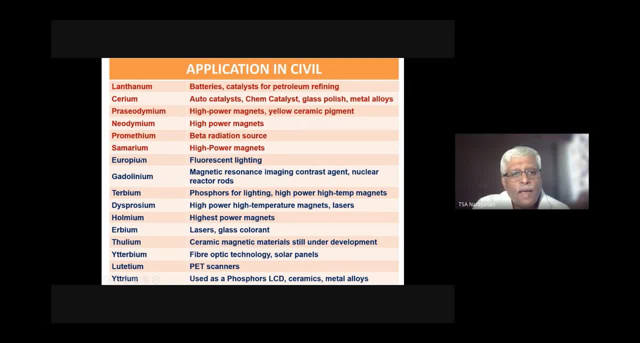 which are in red are available in plenty in india and the balance which are available, dark blue- are very rarely available. but these first six which are available in india are the lrre. that is the content. they are low rare earth elements, so extraction process is much more difficult. you can. 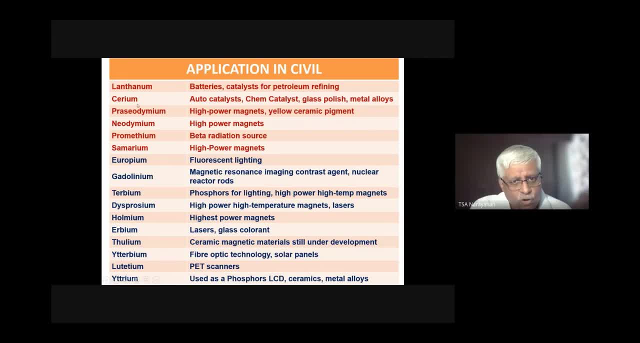 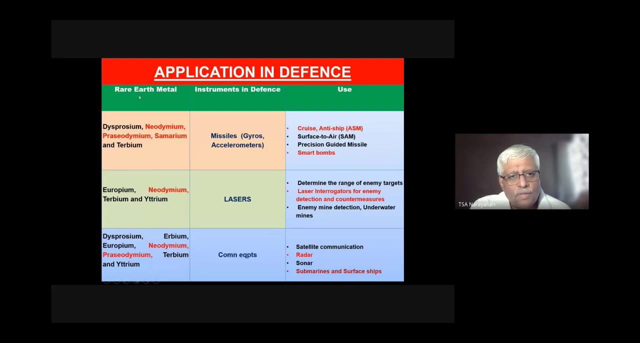 see where all they used. i already covered them. but if you want to see individually these rare earth elements, how they are each in elements, how they are utilized, in which all industry is given, in these slides coming to application and defense, i have divided into three columns. first column is: what are the 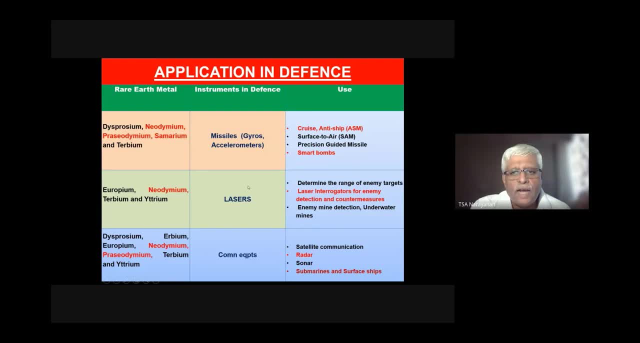 rare earth metal. what are the instrument in defense and in which part it is utilized. so that is what it gives. so if you look at the rare earth metal- dysporium, neodym, prosodium, samarium and terbium- this is: these are used in gyros and accelerometers, which are further used in anti-ship. 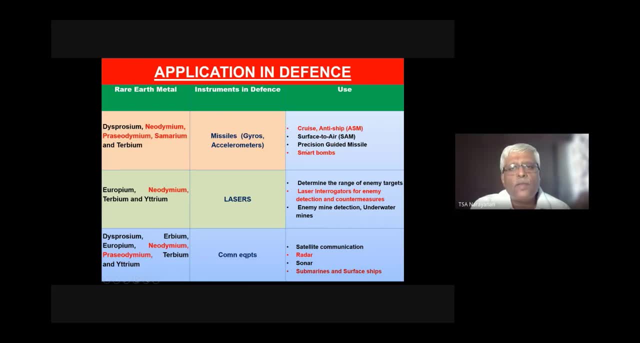 cruise missiles, surface to air missiles, precision guided missiles and smart bombs. the europium and neodym terbium and uterium rare earth are used in lasers for determining the range of enemy targets. laser integrators for enemy detection and counter measures, enemy mine detection and underwater mines. the dysporium erbium, europium, neodym prosodium. 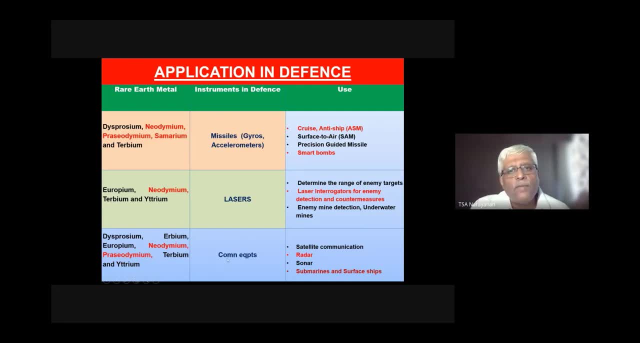 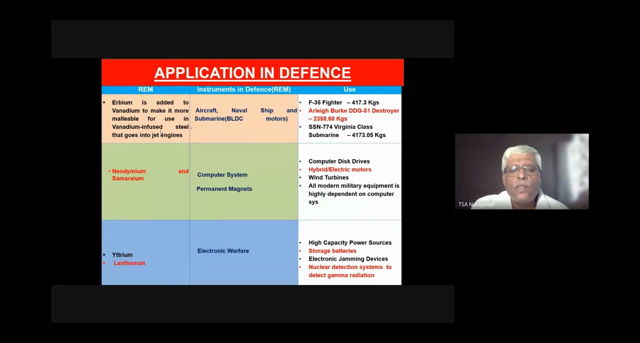 terbium and uterium. they get utilized in the communication equipment for satellite communication, radar, submarine and surface ships. now if erbium- it's one of the rare earth- is added to vanadium, which is a metal, to make it more malleable for use in vanadium infused steel that goes into jet engine. 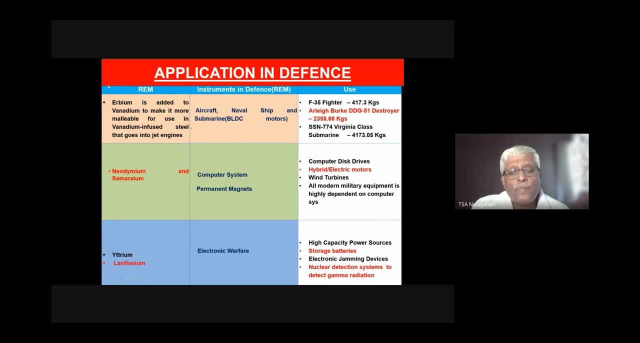 which gets utilized in aircraft and naval ships and submarine. you'll be surprised to know that the f-35 fighter, which the usa, you know, brings out every now and then, has got 417 kg of radar. their air leg bucket destroyer has got approximately 2300 kgs of wearer, their ssn. 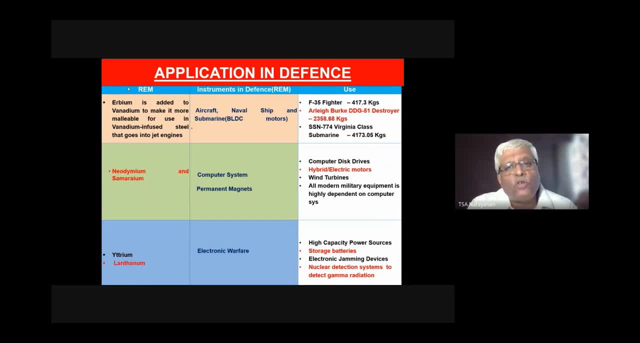 virginia class submarine has got approximately 4000 kgs of weather. so this kind of rare earth is used in our ships, in our fighter aircraft also. those figures are not part of the public domain. neodym and samariums are used in the computer systems or in permanent magnets, which gets further. 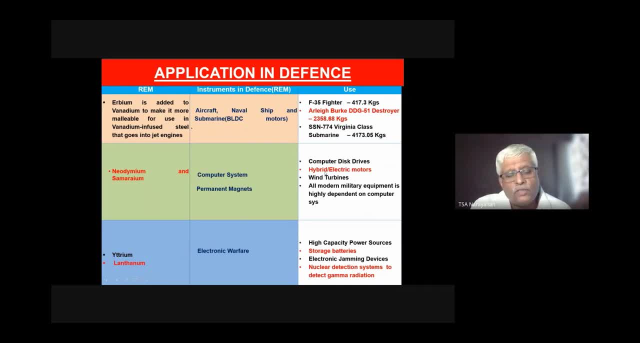 utilized in the computer disk drives, hybrid electric motors, wind turbines and all modern military equipment which are highly dependent on computer system also use them. the yttrium and lanthanum, which we have large numbers in india, are used in electronic warfare. it could be the high. 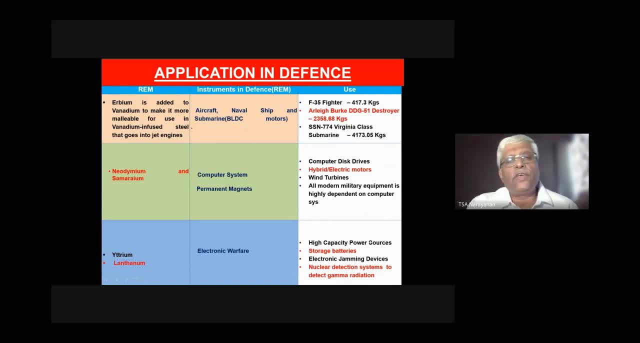 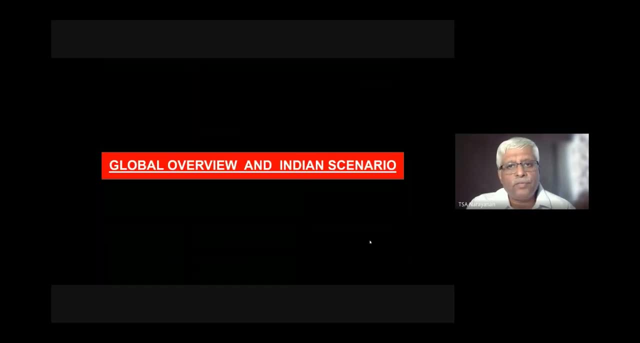 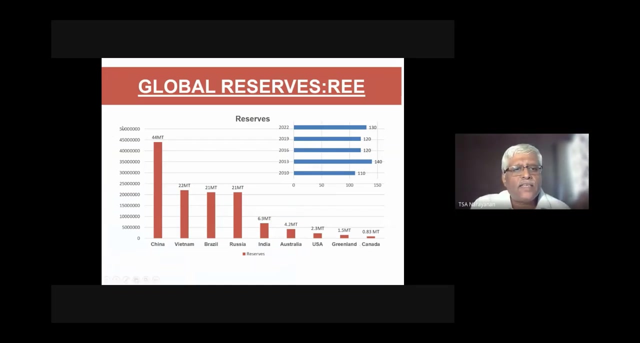 capacity power source, in storage batteries, in jamming device and also used in nuclear detection system to detect gamma rays. now, looking at that, after seeing how this radar gets utilized, let's look at the global overview and the indian scenario. if you look at the global reserve of rare earth, the y-axis gives the 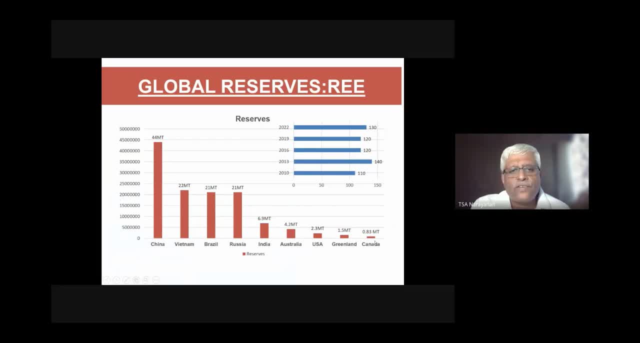 approximate tonnage and accesses the countries. if you look at china, china has got 44 million tons as global reserves of his own reserves of rare earth. india has got 6.9 million tons, which is more than australia and usa. now, if you look at the total reserves of the earth assets, 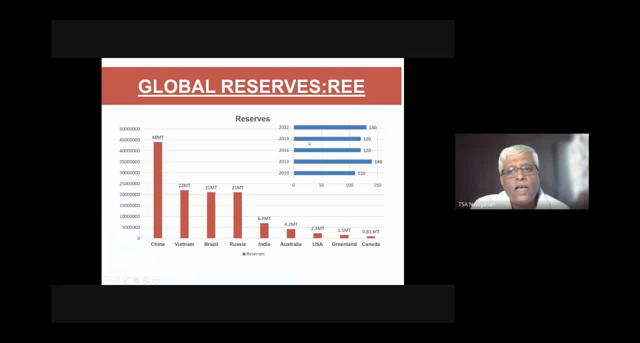 in 2010 we had 110 million tons and in 2020 we have 130 million tons. so, if you can imagine, 130 million tens, whereas gold was only 2.1 lakh tons and we are so crazy about gold. so the availability of rare is plenty and the availability of rare earth is higher than. 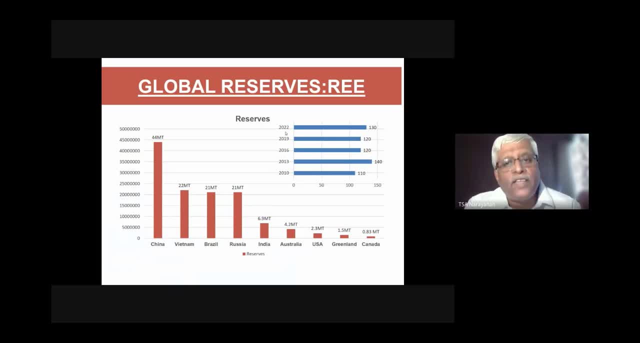 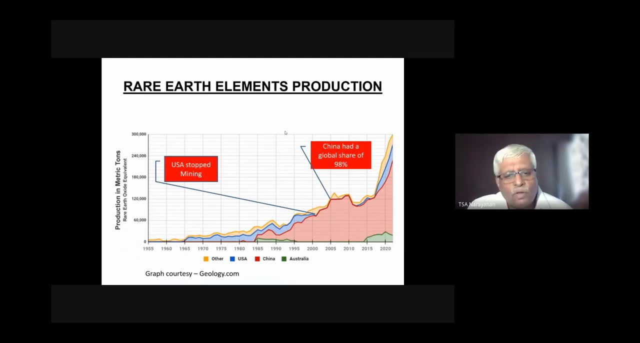 and is in plenty in india itself. 6.9 million tons is another slide, which gives you a little bit. you know how the rare earth came about. so this graph- actually the y-axis gives you the tonnage, production year by year and the x-axis gives you the year. the yellow line depicts others, the blue line depicts usa. 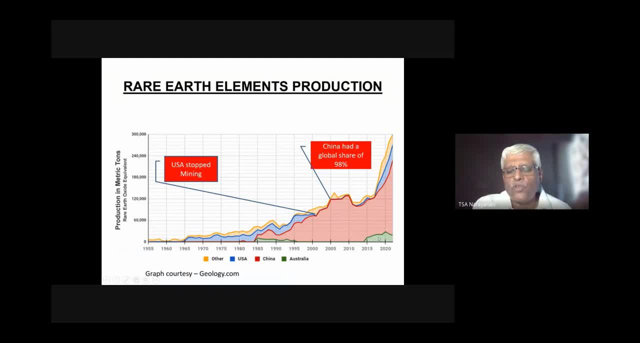 this red portion is china and this green portion is australia. now, if you look at it, this mining of rare earth was started by usa company in 1965 and some other countries are also producing it somewhere. in 1983, china entered this business, subsidized all its factories and started pumping rare earth at very cheap rates. 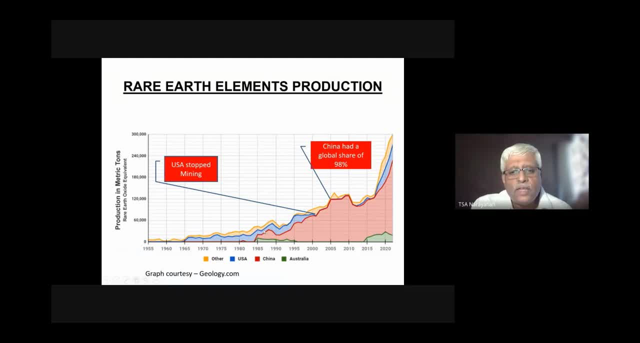 into the world. you look at this. suddenly the production of usa started decreasing and somewhere in 2002- 2003, the usa stopped mining because it was not economical. so at that time only china was a major rare earth producer, and in somewhere in 2005 china had a. 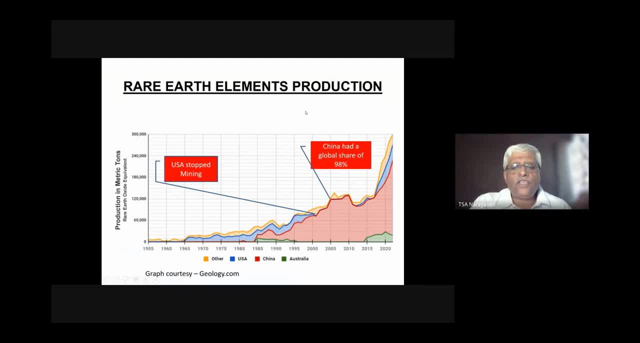 global share of 98 percent. this once it had a 98 percent somewhere in 2011-12. china put a little bit of a ban. i will put it: reduces export to especially western countries. for one thing, they didn't want this ex western countries to develop their own technology using rare earth, so just reduce the. 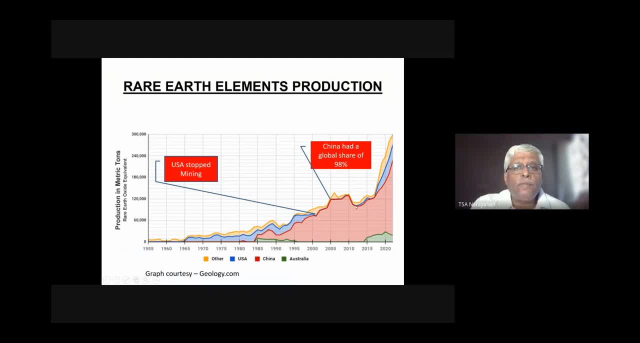 export, due to which the america started producing its own rare earth again in 2013, and you can see this blue line coming up today also. china controls 70 percent supply of rare earth to the world and does about 14 percent of the error up to the world, and balance is by the rest of the world. 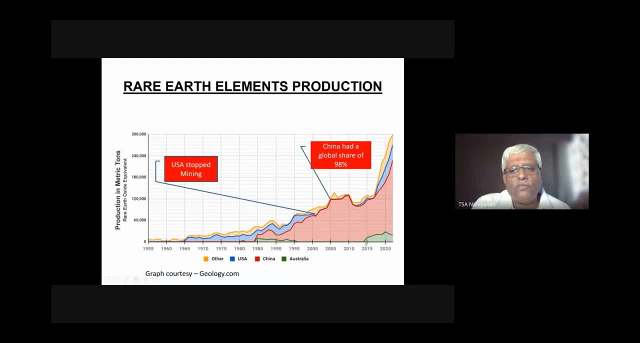 you can see the bottom. australia has suddenly taken off somewhere in 2014 and is one of the major supplier. it has become remember. australia has got less reserve. australian usa has got less reserve than india, but is producing much, much more than india. this is another graph which will make it. 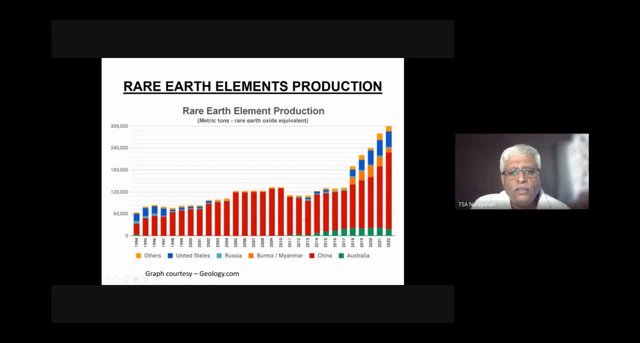 easier for you to understand the difference between the two countries, and you can see in the chart here: this red depicts china, blue is usa, cyan is russia, yellow is others if and green is australia. if you look at it again, as i said somewhere, in 2003 usa stopped and after that china. 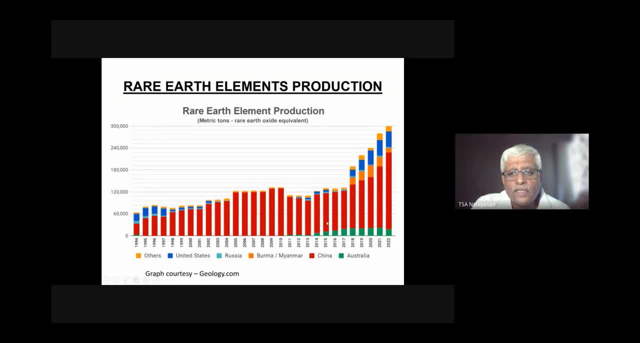 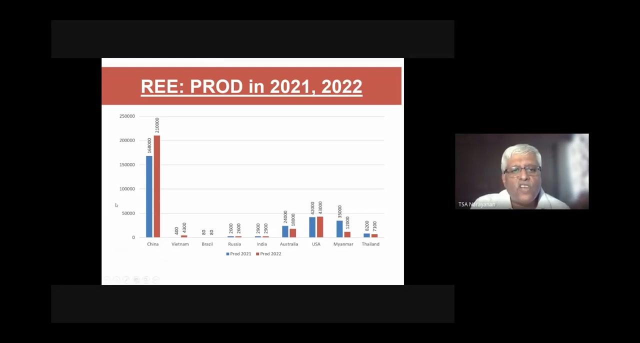 took over and somewhere in 2013, usa also once again entered. but the best part is somewhere the big way. and burma, which has got less reserves, has got more production capacities than india. similarly, australia, which is in green, has got more production capacity than india production in 21 and 22, just to say. where are we recently? china is still dominating with about 2. 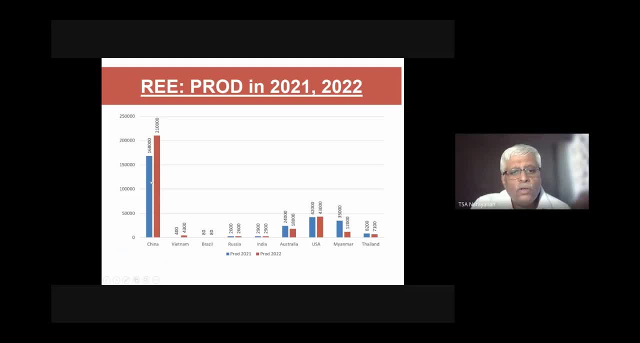 lakh 10 000 production in the year 22.. then next comes usa with 43 000 production, then australia, thousand. india is very low. production is only 2900 tons. russia is also 2600 tons. here it is myanmar. myanmar last year produced 35 000 tons and last year wins when i say is 21 and in 2022 it produced. 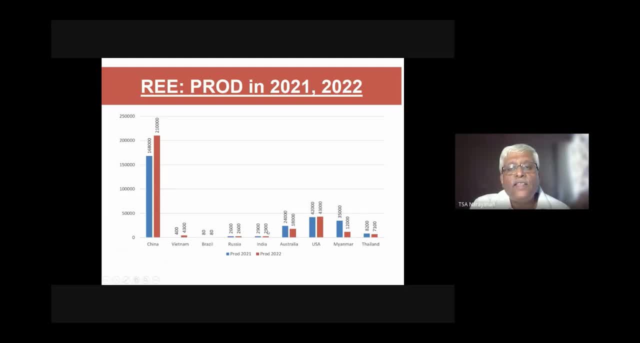 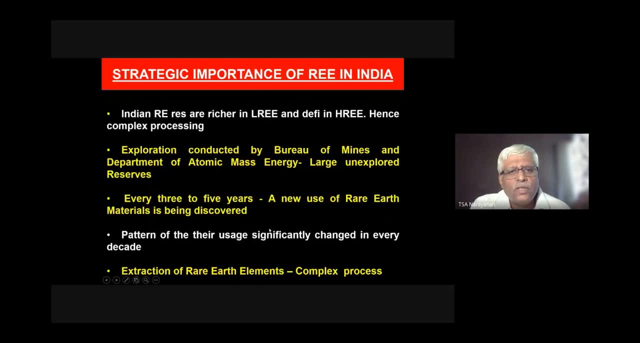 12 000 tons, much, much higher than india, whereas the reserves are less there. now, what are the strategic importance of rare earth for india? as such, india reserves are richer and more efficient and deficient in higher rare earth elements, hence complex processing which i told you before. exploration is conducted by bureau of mines and department of atomic mass energy. this 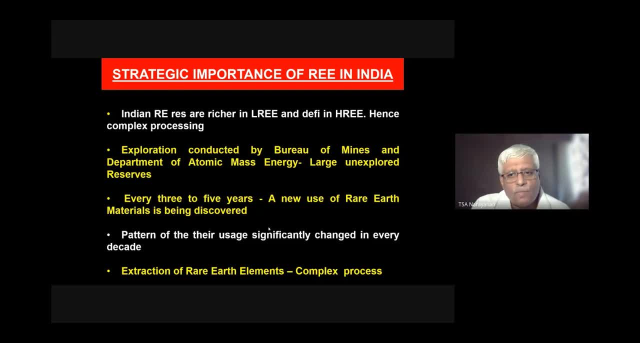 bureau of mines comes under the department of atomic energy. we have large unexplored reserves exploration. this is costly. every three to five years a new use of rare earth material is being discovered. the pattern of the rare earth is the same as the pattern of the rare earth material is. 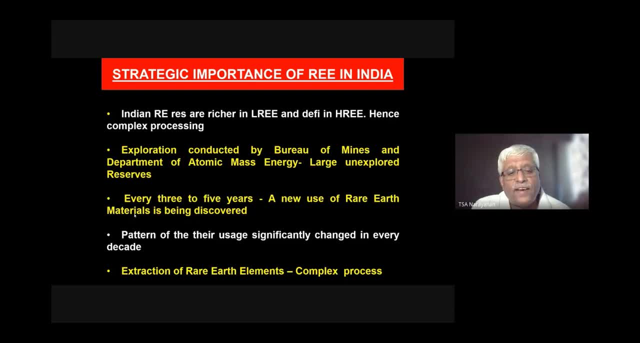 being discovered. the pattern of the rare earth material is being discovered. the pattern of the rare earth changed significantly in every decade. 1962, the color tv first time came. the rare earth got utilized and rare earth was commercially utilized in a big way. today rare earth is used. 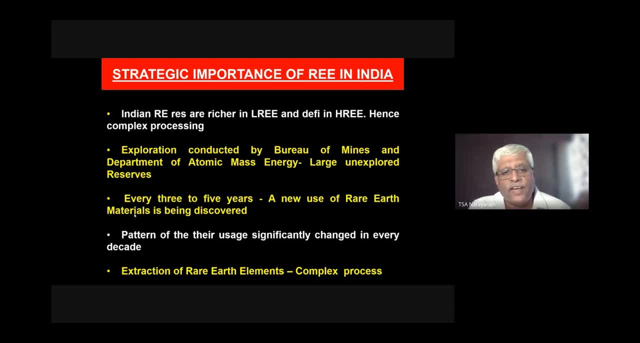 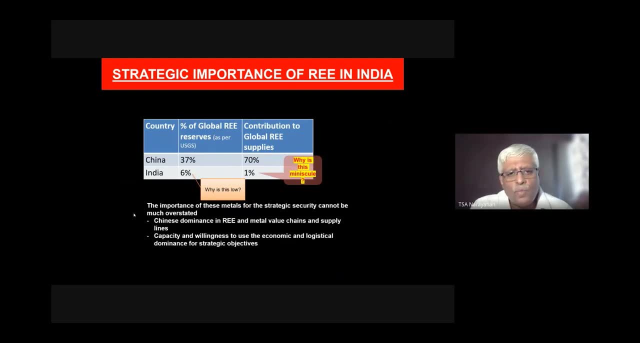 in military equipment usage keeps on changing every decade. extraction, as i said, is a very complex process. now, if you look at this slide, this slide, the column first gives you the country it says the percentage of global reserves and contribution. china, which is, has 37 percent of. 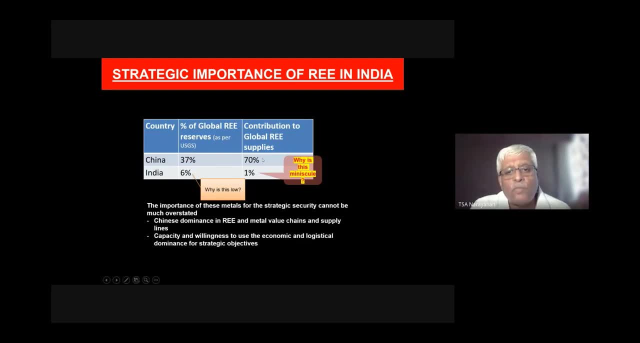 global reserve is contributing to 70 percent of production every year. india, which has got six percent of the global reserve, is contributing only one percent of production or supply to the world. this is how the china is able to dominate the rare earth element and is able to put 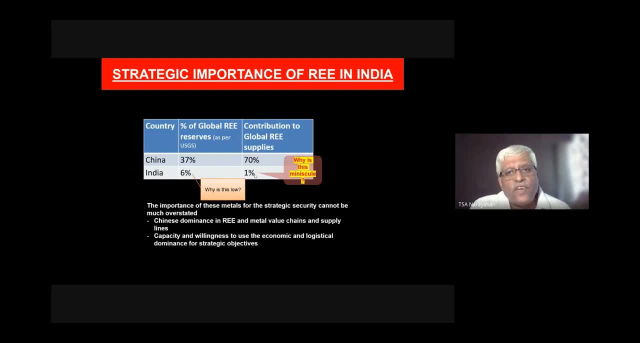 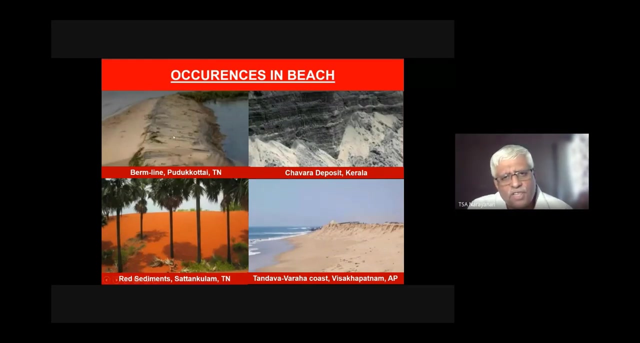 value in supply chain. this is where india has to use economic and logistic for strategic objectives by ensuring that we invest in rare produce, more, export more. start making rare earth permanent magnets. now, where does it occur? in india? it occurs in most of the beaches which have got manzanite. it occurs 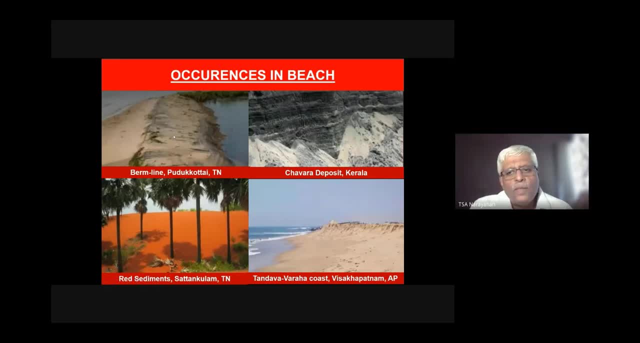 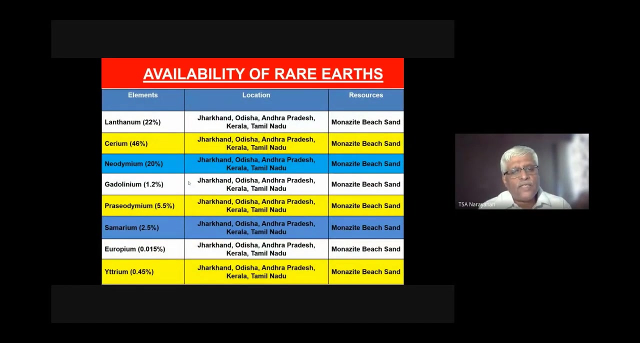 there, for example, in pudukota, tamil nadu, a chawara deposit, in kerala red sediment in tamilnadu, in santa sataniculam, in tandara barra coast, in vishakhapatnam, andervadesh, and this is i'm listing it out. the first column gives you: 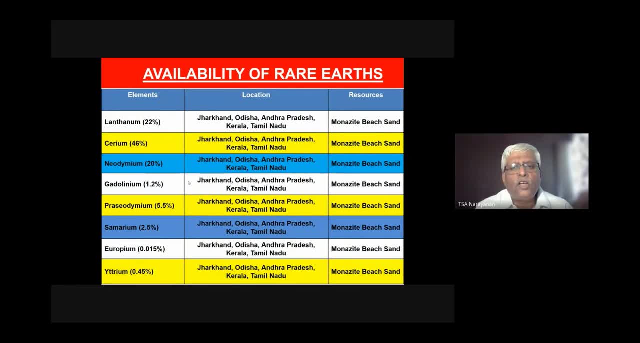 the element locations are generally the same. the resources are same, which is the third column. what i have written is a percentage. if hundred percent rises, if we take twenty two percent of lanthanum is held by india. this renovation is yielded to Kong want at 72 percent of lanthanum is held by india, but 600 percent, 72 percent is current. seventh percent of aljali produce as conserved land: ian. 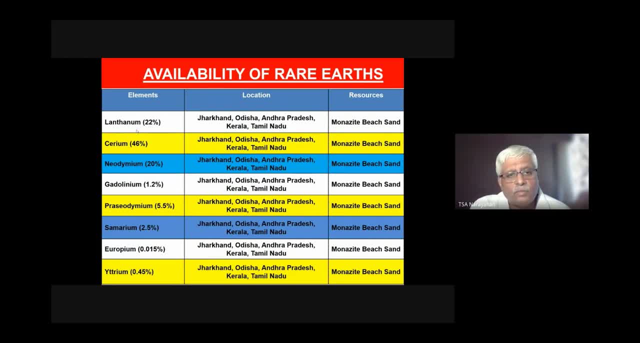 India, 22% of rare earth is lanthanum. Cerium is 46%. Neodymium, which is used for making permanent magnet, is 20%. Like that. we have percentage. The first six until samarium are the low rare earth. After that, if you see, the percentage is decreased: 0.8, 0.1.. These 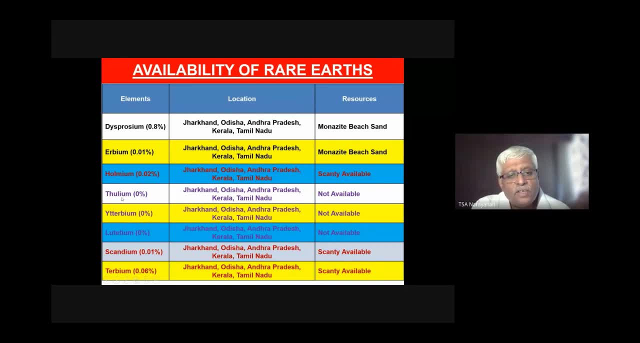 are the high rare earth element And there are three rare earth elements which are just not available in India, which is thulium jetrubium and lutetium And balance are available in many school quantity. There's an extraction process for this rare earth. It's a simple. 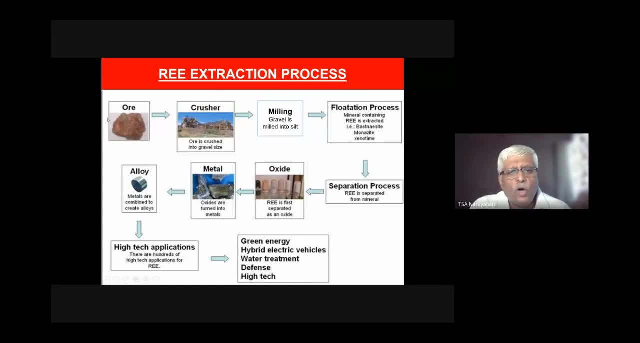 mining process very easy to understand. The ore is crushed into gravel size. This gravel is milled into silt. Flotation process is used so that REE could be extracted- monzonite. Then the REE is separated from mineral. 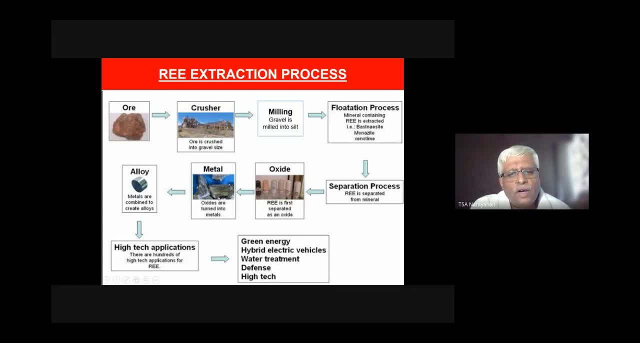 They are oxidized and then they're turned into metals. These oxidates are turned into metals and into alloy and then used in for high-tech application. where they're generally used is in the green energy, hybrid electric vehicle, water treatment defense technology. 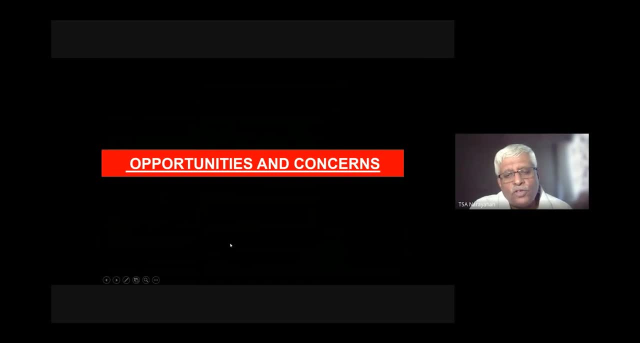 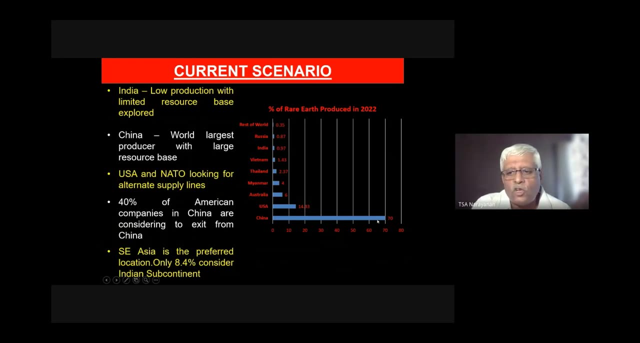 and high-tech technology. Now, what are the opportunities and what are the concerns? The current scenario, as I told you, this grass gives you the percentage contribution of rare earths by each country. You can see: China is 70%, India is 0.97, is approximately 1%. 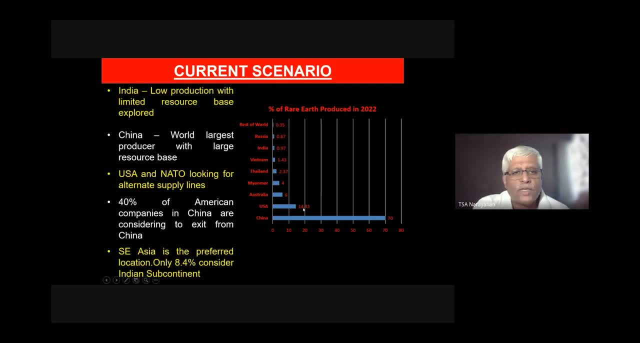 And USA is 14%. The second column is USA. India has got a low production with limited resource base. explode China, world largest producers with large resource base. USA and NATO are looking for alternate supply lines. 40% of American companies in China are considering. 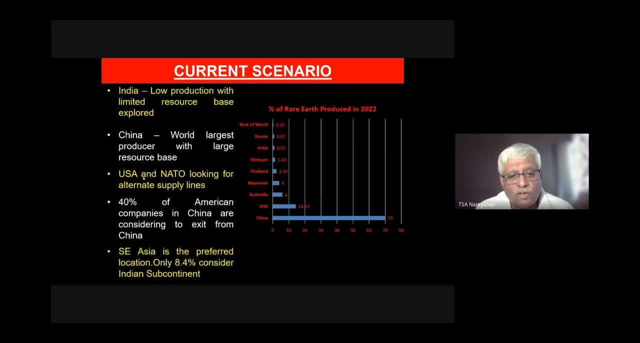 to exit from China. This is a big problem. So we're going to have to wait and see. We're going to have to see what happens, We don't know. So we're going to have to let this process go and hopefully we'll have a huge opportunity for us. But unfortunately, Southeast Asia that. 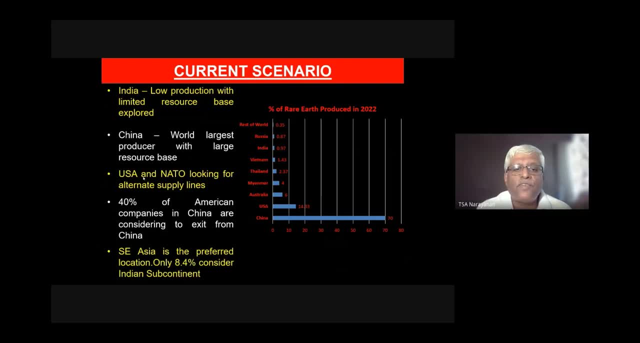 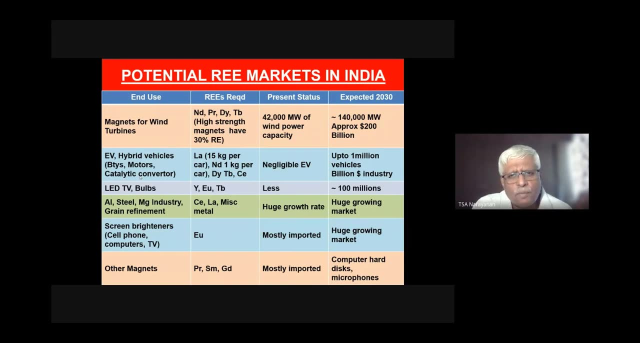 is Malaysia, Vietnam, Thailand. these are the preferred location. Only 8.4% considered Indian subcontinent. Now what are the potential market assets in India? The magnets for wind turbine, where this neodymium, trisodium, diptyprodium and trubirium is utilized. 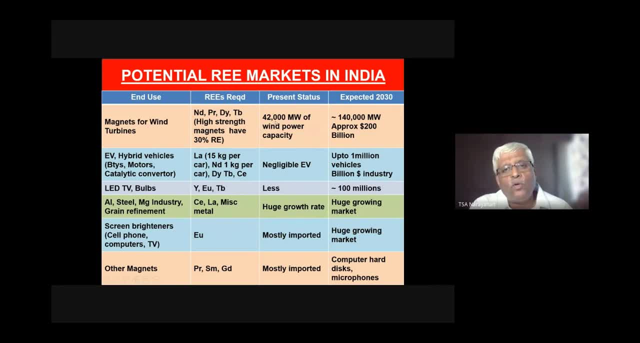 Present status, you are able to produce 42,358 touchingepčr. That is a very small amount: 000 megawatt of wind power. today. it is expected to go up to 1 lakh 40 000 megawatt power approximately. 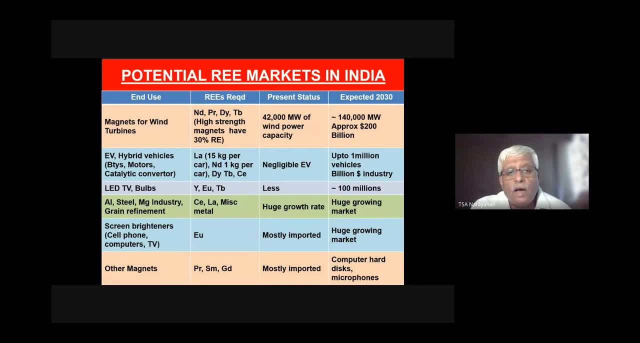 200 billion dollar business is going to be. imagine the amount of rare earth which is going to get utilized here- about 30 percent. is there utilization in the electric vehicle, in the hybrid vehicles, used for the motors, catalytic converters and other thing? lanthanum: approximately 15 kg per car. 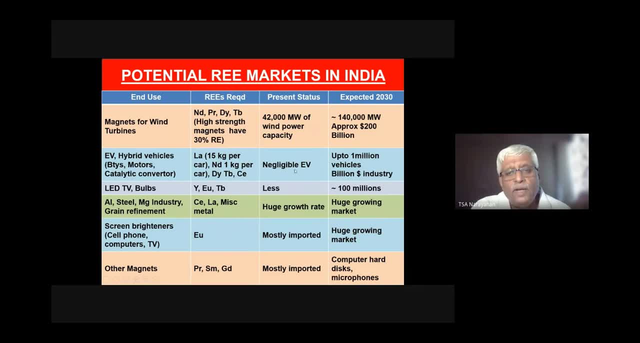 neodymium, 1 kg per car today. i say negligible electric vehicle compared to petrol and diesel vehicle, but up to 1 million vehicle will get sold every year. it's a billion dollar industry. similarly, led tv wells today. the present status: yes, we have expanded, but scope is it's going to? 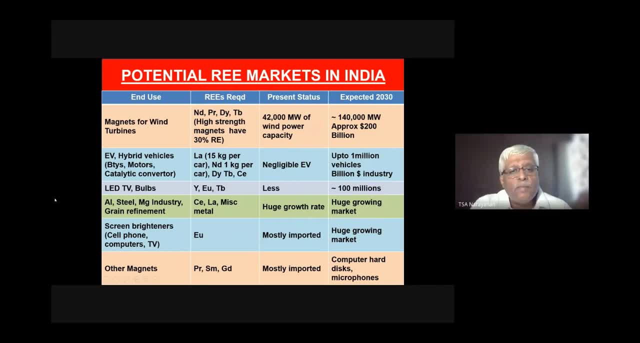 go to 100 million every year. aluminum steel, manganese, grain refinement- huge growth rate and a growing market screen brightness, basically for cell phone computers and tv, europium. these are mostly imported. it has got a huge market, even anyone who's making mobile or tv. and in other magnets also prosodium samurium is utilized and these are mostly imported. 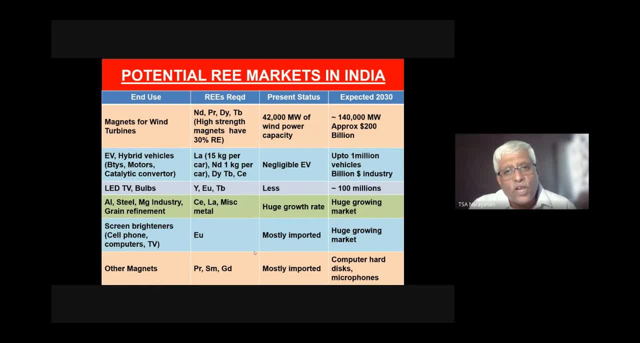 used in the computer hard disk and in microphones. so there's a potential market. so if we grow our rare earth and produce sufficient, we will have the capacity to absorb them. we will need not import them. plus, we will be able to export and earn some foreign exchange. 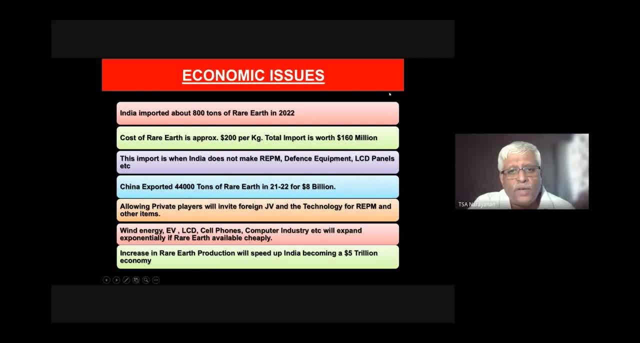 yes, as i said, foreign exchange. coming to the economic issues, india imported about 800 tons of rare earth in 2022. i mean, you will say this is not much- 800 tons. you are also producing approximately 4 000 tons every year. today, let me tell you, we are not manufacturing rare earth. 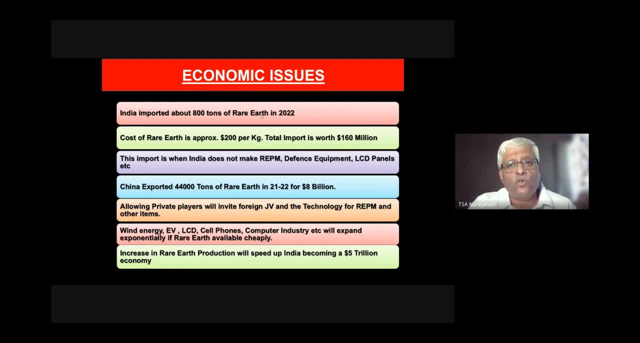 permanent magnets which are used in electric vehicles, which are used in motors, generators and other equipment which is. we are also importing this. if you can not only make rare permanent magnet, it will all get utilized in your wind turbines, in all other magnets where the magnet is used. you will be able to export them also. 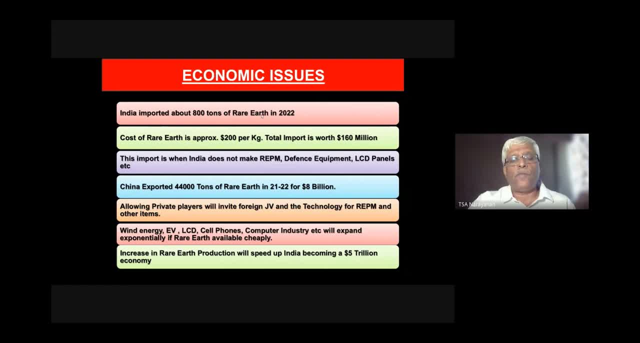 second, we are in atman river. we are making defense equipment. but we are not yet started making defense equipment where large amount of rare earth is being utilized again. same goes to permanent magnet and other parts. so when these things get started producing in india, we will be importing a lot of rare. today, government does not have the kind of funds. 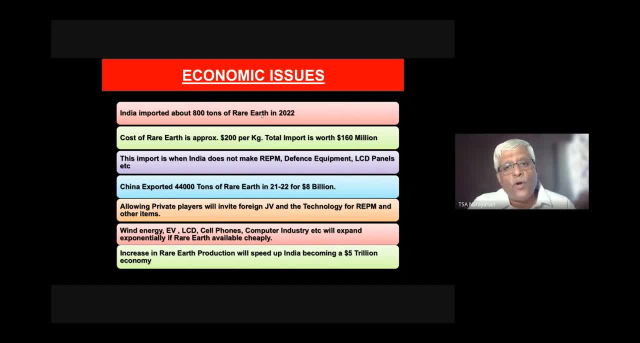 that is needed for exploring this error and for producing. that is why you need- we need to encourage the private sector to come. so, as i said, this import is when india does not make repn. that is a rare permanent magnet defense equipment, lcd panels. china, last year exported 44 000 tons of. 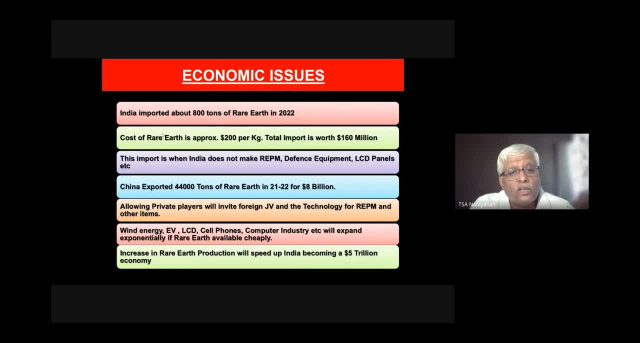 error for approximately 8 billion dollars. the allowing for private players will invite foreign jv and the technology required for rare permanent magnet and for other items: wind energy, electric vehicle, lcd, cell phones, computer industry will expand exponentially if rare earth becomes cheaply available in india. it will be if 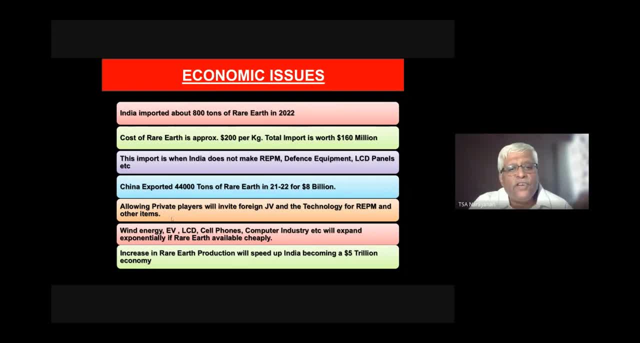 we explore more, we produce more. increase in rare earth production will speed up india becoming a 5 trillion economy, because we will be not only will be able to make rare permanent magnet and other items, we will be able to export more and tap into this 8 billion which china is making. 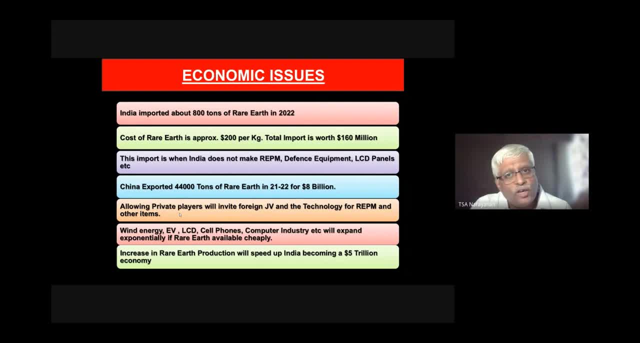 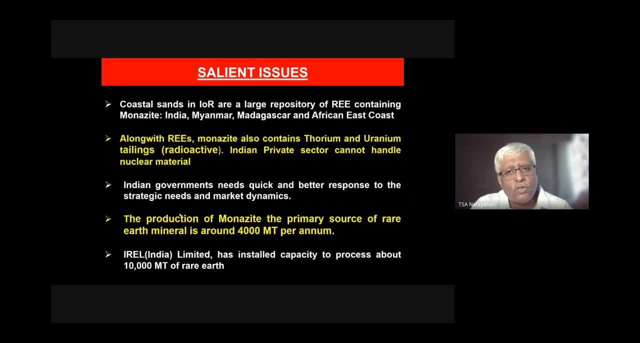 we will also be able to take something out of it- and is only going to increase the usage of rare earth. is only going to increase and not decrease. some silent issues with respect to rare earth. with respect to india: coastal sands in indian ocean region is a large repository of 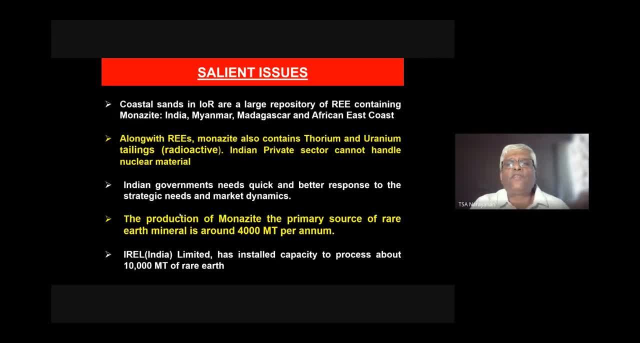 elements containing monsite one side is the basics on which from rare earth is extracted. the country is affected in ior india and african east coast also. along with rare earth elements, monsonite also contains thorium and uranium tailings which are radioactive. indian private sector cannot handle nuclear material. this is one of the basic reason. 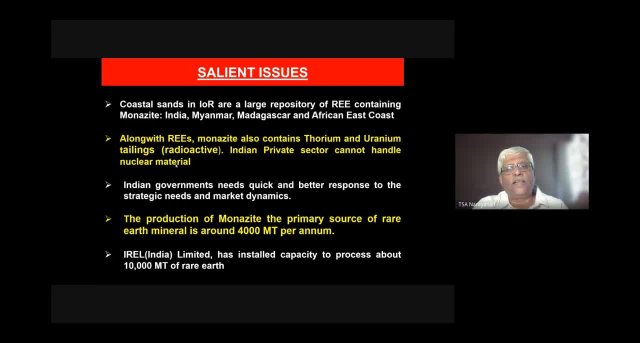 why the government is not allowing the private sector to enter this rare earth element industry. why, because of the mencion of rare earth elements, they do not have nuclear material. and they are not because when you process this manzanite, you are going to get thorium and uranium as side. 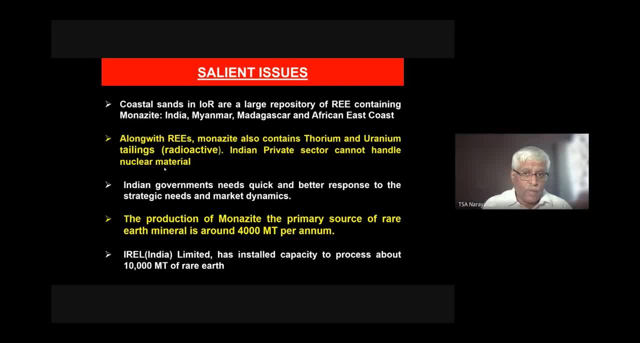 elements of rare earth, but because the opportunity is there, indian government should do a quick and better response to the strategic needs and market dynamics, because this rare earth is going to get utilized in a big way and this is an opportunity for india. today in india, mineral is the monzite from which we are making and our capability is four thousand. 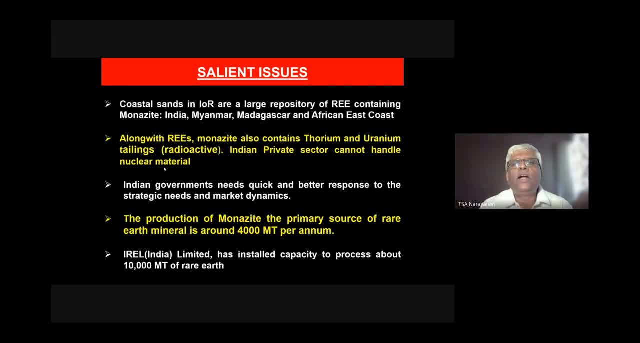 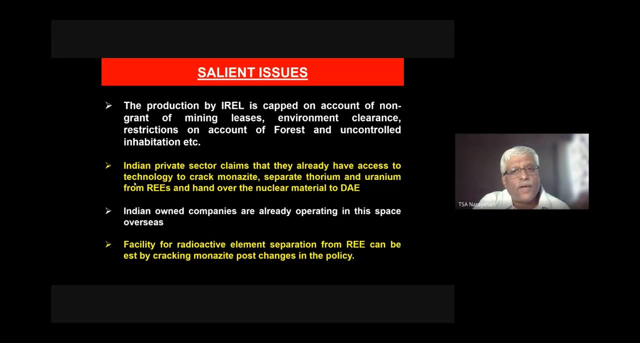 mil and capability producing four thousand tons per annum, but our capability is ten thousand tons per annum. we have the capability but we are producing only four thousand. capability facility for separating this radioactive elements from rare earth element can be established by cracking monzonite. post change the policy, the government india will have to comment. 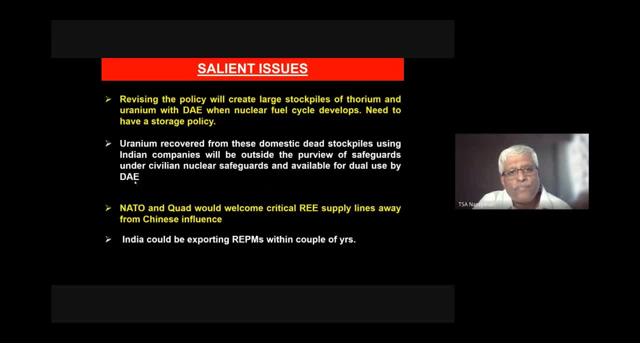 of india will have to change the policy which is existing today. revising the policy will create large stockpiles of thorium and uranium with the department of atomic energy. when this nuclear fuel cycle develops, need to have a storage policy uranium recovered from these domestic dead stockpiles. using indian companies will be outside the 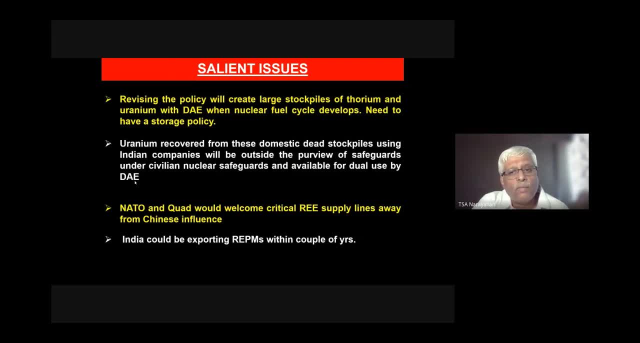 preview of safeguards under civilian nuclear program and will be available for dual use by department of atomic energy. necto and quad would welcome critical rare earth element supply lines away from chinese influence, and india could be exporting rare earth permanent within a couple of years if the policies change and the private players are allowed to come. what 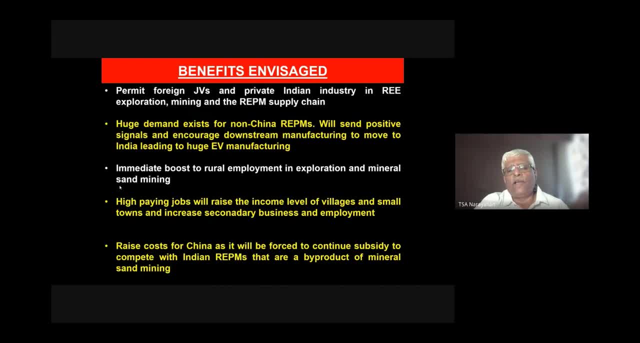 are the benefits we will get if we get into the riders in a big way where we allow the private sector to come first of all, we will get foreign jvs. they will come and they will be attracted toward the private indian industry for exploration, mining and, in rare earth, permanent. 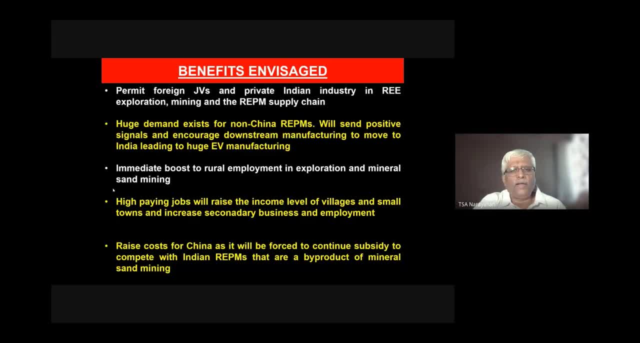 manufacturing and supply chain. huge demand exists for non-china rare earth permanent magnet. will send positive signal and encourage downstream manufacturing to move to india, leading to huge ev manufacturing. immediate boost to rural employment in exploration and mineral sand mining. high paying jobs will raise the income level of village and small town and increase secondary business and employment. 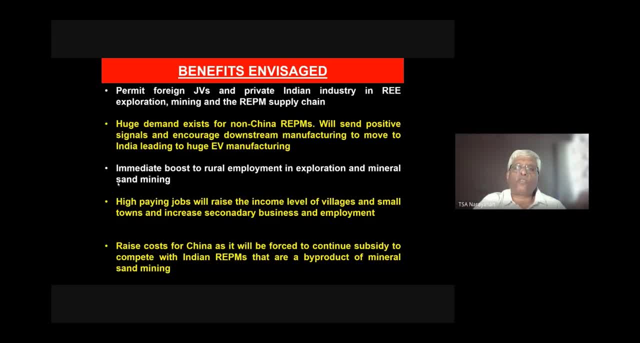 this will also raise costs for china as it will be a major part of the development of the rural development of rural development in rural areas and the development of rural development in rural areas will be forced to continue subsidy to compete with indian rare earth permanent magnets that will be the byproduct of mineral sand mining, green power technology. 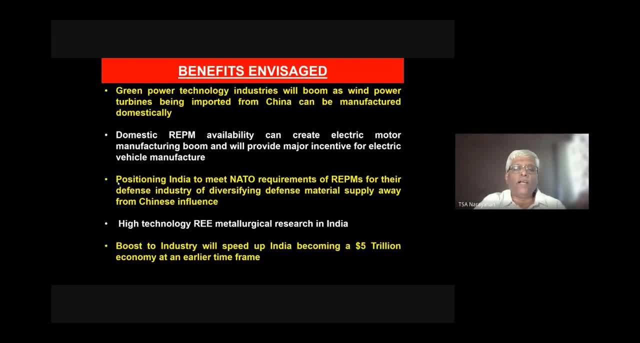 that is, windmill industry will boom as wind power turbines being imported from china will be manufactured domestically. domestic rare earth permanent magnet availability can create electric motor manufacturing boom and will provide major incentive for electric vehicle Positioning India to meet NATO requirement of rare earth permanent magnet for their defense. 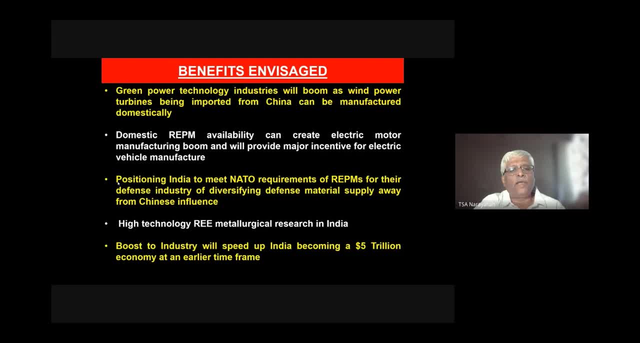 industry and diversifying defense material supply away from Chinese influence will also be beneficial. High technology, rare earth element metallurgical research in India will improve and will get better products. This boost to this industry will speed up India becoming a 5 trillion economy at an. 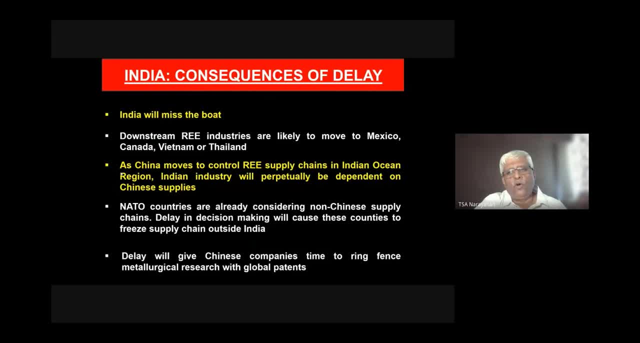 earlier time frame. Suppose we don't and we continue the policy, similar what we have now and no change in policy is done, what will be the consequence of delay? India will miss the boat first. The downstream rare earth industries are likely to move from China to Mexico, Canada, Vietnam. 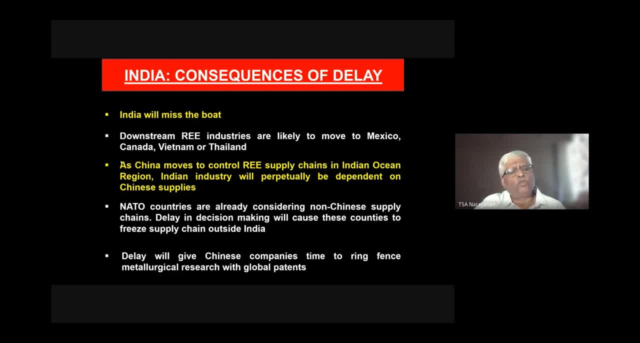 or Thailand. As China moves to control rare earth element supply chain In Indian Ocean region, Indian industry will perpetually be depend on China, or NATO countries are already considering non-Chinese supply chains. Delay in decision making will cause these countries to freeze supply chain outside India.